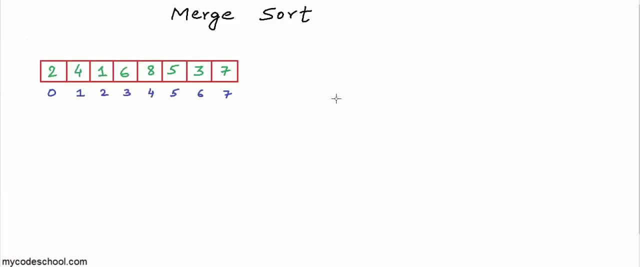 Given a list of integers in the form of an array, something like this: let's name this array a. we have eight elements in the array, So we have indices from zero to seven. we want to sort this list in increasing order of the value of integers, So the list should be rearranged like this: Our approach in merge sort algorithm will be entirely different from what we had done in previous sorting algorithms, where we were rearranging the 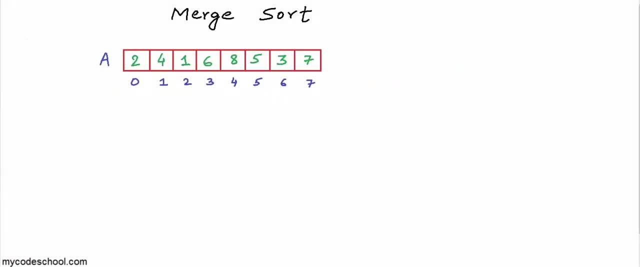 elements or changing their positions only by swapping or shifting. what we are going to do here is we are going to break this problem into sub problems. we will divide this array into two equal halves, or rather two possibly equal halves, So we will find some middle position and we can say that all the elements before this position belong to the first half and all the elements after- on or after this position belong to the second half. If an array would have odd number of 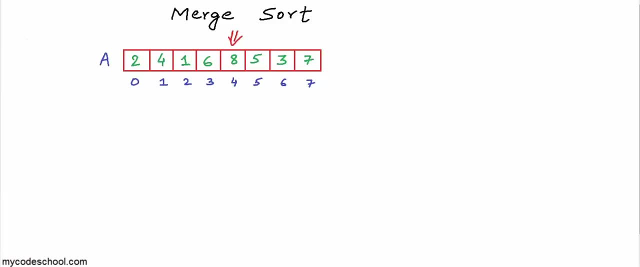 elements, elements. one of the halves will have one more element than the other half. we have eight elements in the original array here, So we have two equal halves. Now think about this: what if we are somehow able to sort these two halves, And let's say these two? 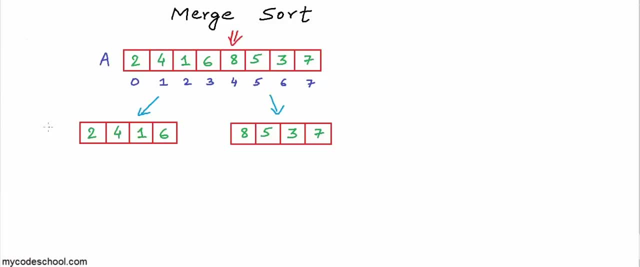 halves are entirely different arrays. they are created separately in memory by copying values from the original array. If we are somehow able to sort these two arrays, then we can merge these two lists together into the original list, in sorted order Of course. 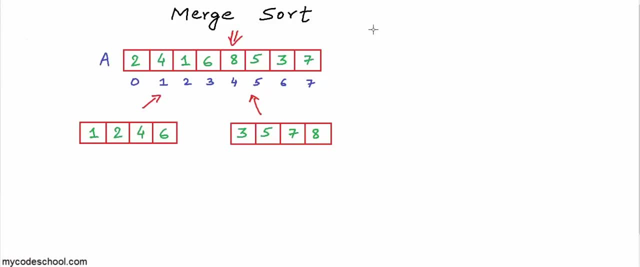 there has to be some algorithm to merge two sorted arrays into a third array, in sorted order. the algorithm will be pretty straightforward. Let's say this particular sub array is named L and this particular sub array is named R- L for left and R for right, Because all 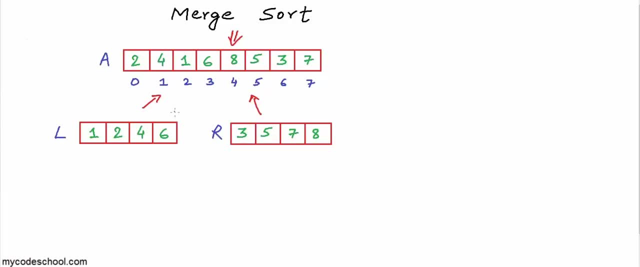 the elements in a are present either in L or R. We can font published on the style index. som mínimum of option m is the best solution. We can start S Dom Adoptionairstxt for the following introduction: The search function. start overwriting A from left to right. We can start with 0th position in A At any point. 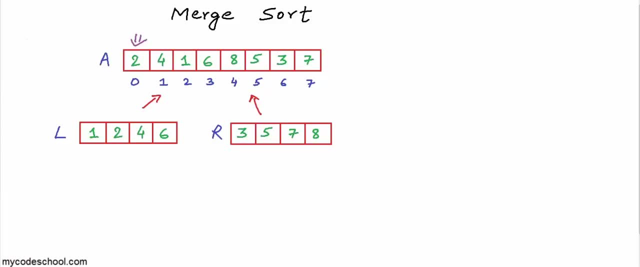 the smallest element will be either the smallest unpicked in L or the smallest unpicked in R. And let's say we color code the smallest unpicked in L and R by this yellow color. What we can do is we can pick the smaller of the two smallest unpicked in L and R. We 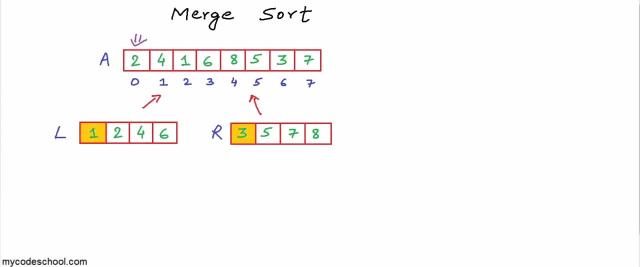 have two candidates here, 1 and 3.. 1 is smaller, So we can write 1 here at 0th index and now we can look for the number to fill at 1th index in A, Let's say the cells of the picked. 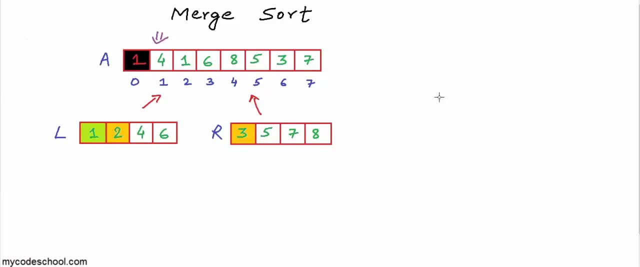 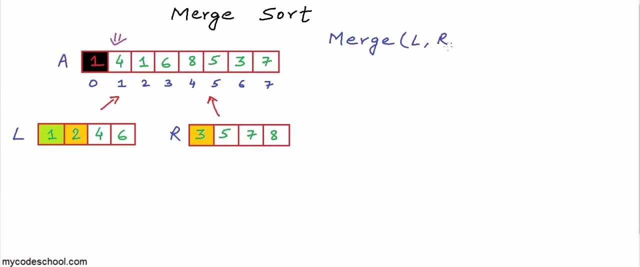 elements will be color coded in green. If I have to write pseudo code to merge the elements of two sorted arrays into a third array. let's say we want to write a function named merge that will take three arrays as argument: left, right, And the array in which it should be merging the two sorted arrays left and right. Then 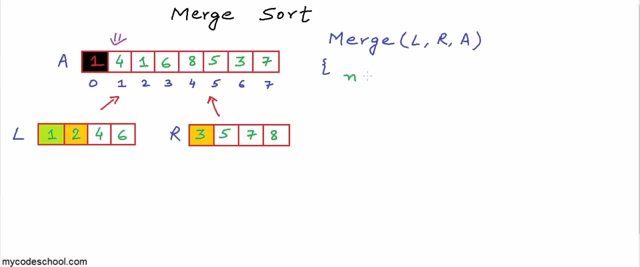 I will do something like this. I will first take a variable that will store the number of elements in L and another variable that would store the number of elements in R. In a real program we can also pass these two values to the function. Now I will take three. 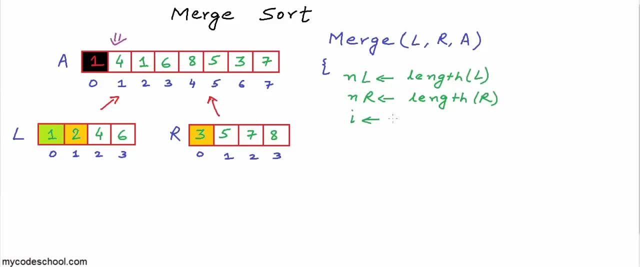 variables i, j and k and initialize them all to 0. Let's say i will merge the two sorted arrays. So i will mark the index of the smallest unpicked in L, j will mark the index of the smallest unpicked in R and k will mark the index of the position that needs to be. 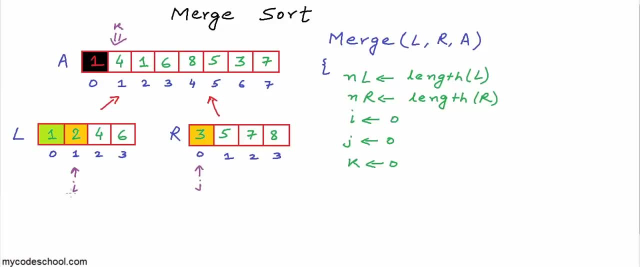 filled in A. For our example. here at this stage we have i equal 1, j equal 0 and k equal 1, because we have already filled one element at index 0 in A. But when we will start, we will start with all three: i, j and k. So we will start with all three: i, j and. 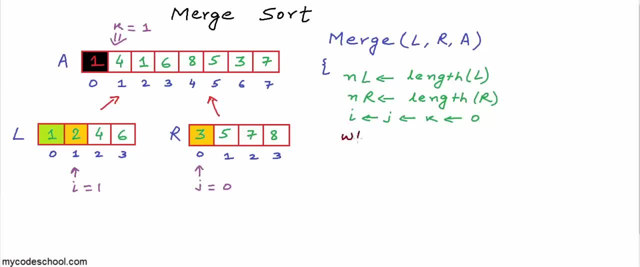 k as zero. And now my code will go like: while i is less than n L, If n? L is the number of elements in L, then for i to be a valid index, it should be less than n? L, And similarly, for j to be valid, it should be less than n R. So while both, 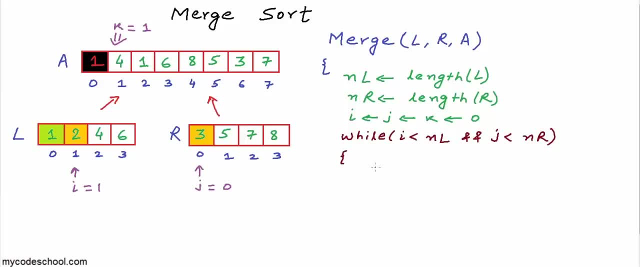 these two indices are valid. both these indices, i and j, are valid. we can say something like: if li is less than or equal to Rj. So we are comparing the smallest in, or rather smallest unpicked in L, with the smallest unpicked in R, In this case at kth position in A. we will 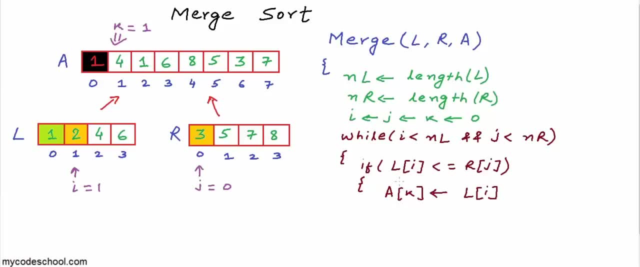 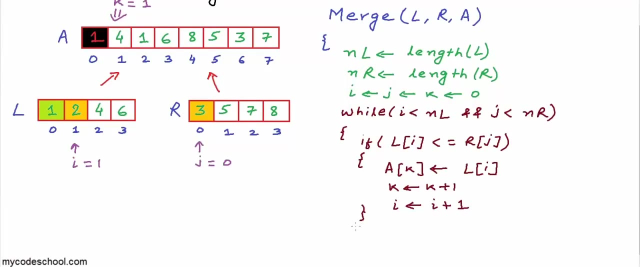 write Li. Remember we are overwriting A and that's not a problem. and now I need to increment k and need to go to the next position, and I also need to increment i to go to the next unpicked in L. and if this condition is not true, if Rj is less than Li, then Ak will be Rj. 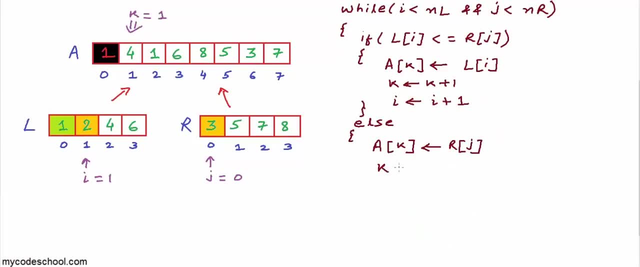 and once again we need to increment k and we need to increment j to go to the next unpicked in R. This k, equal k plus 1, is in both the conditions, if as well as else. so I have moved it out. Coming back to our example here i and j are both valid in D. 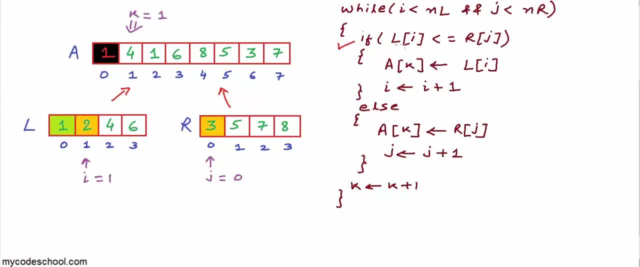 Now we will compare if Li is less than or equal to Rj. Well, yes, Li is less than Rj, so we need to pick 2 for 1th index and we need to increment both i as well as k and for the next position. 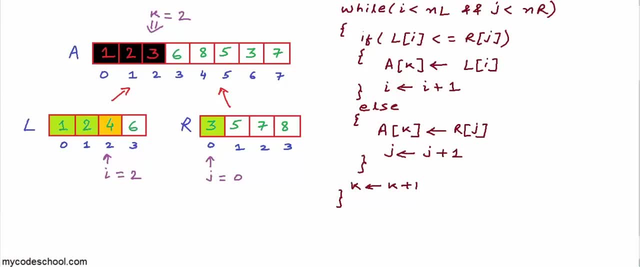 it's between 4 and 3.. 3 will go and we will increment j and k this time. Next it's between 4 and 5.. Next it's between 5 and 6.. Next it's between 7 and 6, and after 6 has gone, we are done with all the elements in L. 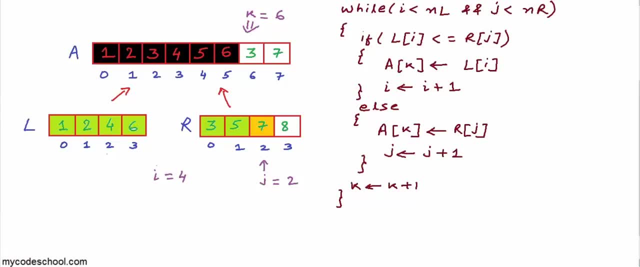 i is equal to 4 now, which is not a valid index. So in the while loop, this condition- while i less than number of elements in L- will be false, and this is definitely one probability. one of the arrays, L or R, will exhaust first. In that case we need to pick all the elements from the other array. 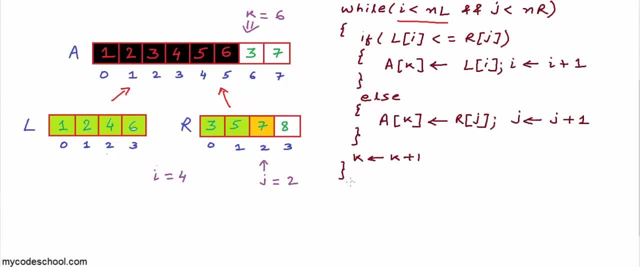 and fill rest of the positions in A. After we come out of this, we need to go to the next position and we need to increment j to go to the next position. For this while loop, we can write statements like: while i is less than the number of elements. 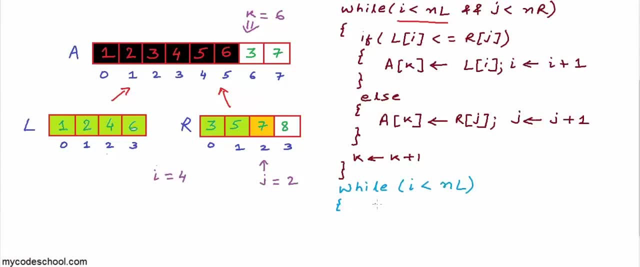 in L, So we can check whether there are left overs in L. We can do the same thing. we can say ak is Li and then we can increment i as well as k. I am short of space here, so I am writing multiple statements in the same line, and similarly we will write a while loop like: 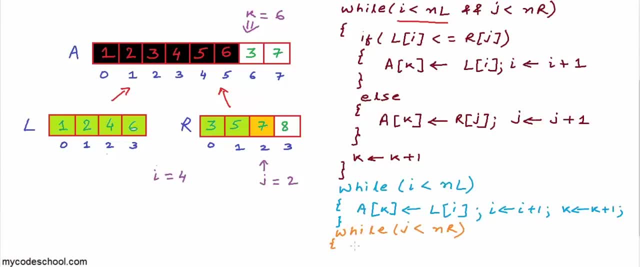 while j is less than number of elements in L, We can fill in ak with rj, and this time j and k will be incremented. Once we are out of this first while loop, only one of these two while loops will execute, because only one of the sub lists or sub arrays will have left overs. For this particular example, this: 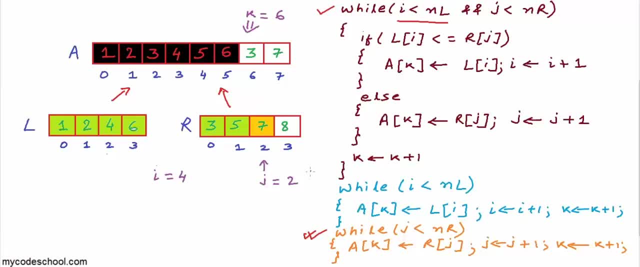 third, while loop will execute because the right sub array has left overs, So we will fill up all the remaining positions And finally, we will have a sorted arrangement in A. This is our merge logic and there are couple of ways in which we can clean up this code further, but for now let's just understand. 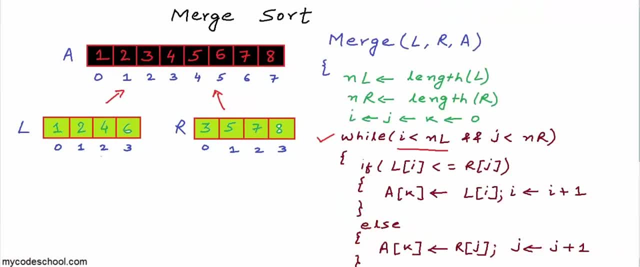 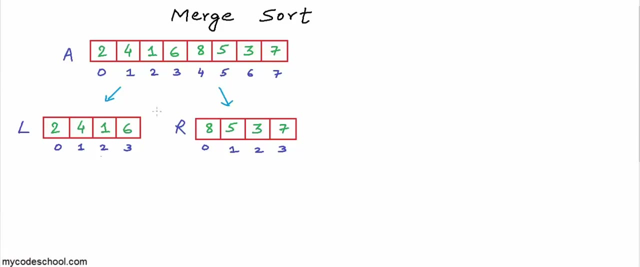 the logic. And now coming back to where we had started, In the beginning we had imagined that if somehow these two sub arrays or sub lists- I am redrawing the unsorted original array and the unsorted array- So we had said that if we are somehow able to sort these two lists then we can merge. 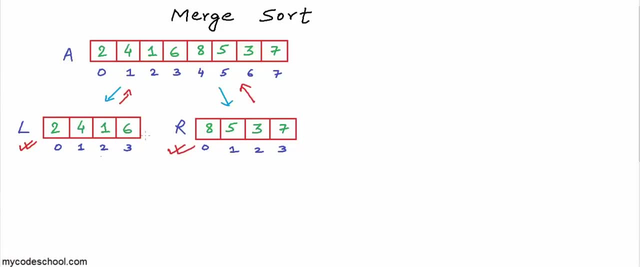 them back into the original list. But of course we need to have a deterministic logic to sort these two sub lists or sub arrays also, And the logic is we can break these sub lists even further. So this sub list comprising of four elements- two, four, one and six- can be further divided. 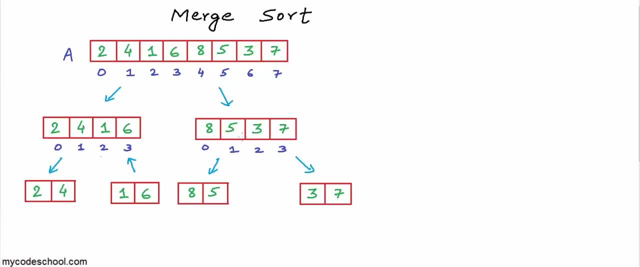 into these two halves and this list comprising of eight, five, three, seven, can be divided into these two sub lists: eight, five and three, seven. The solution for two, four, one six, this particular sub list, can be constructed after we sort these two sub lists- two, four and one six- and merge them back and similarly 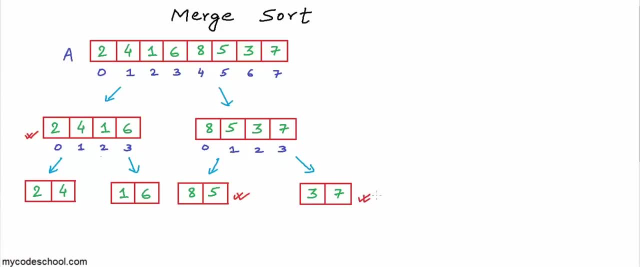 we can sort these two Lists, sub lists, and merge them back to sort this eight, five, three, seven sub list. Once again, we have these four sub lists of two elements each, and they can also be divided. What we are basically doing here is that we are reducing a problem into sub problems in 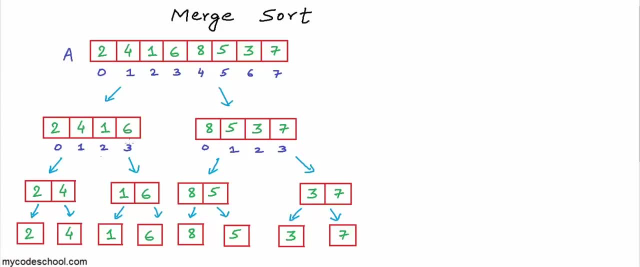 a recursive or self similar manner and at any step, once we get solution for the sub problems, We can construct the solution for the actual problem. If we have two sorted sub lists, we can sort the parent list also. We can go on reducing a sub list, only till we have more than one element in the sub list. 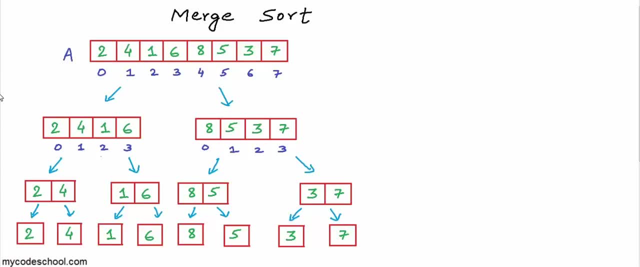 Once we reach a stage where we have only one element in a sub list, then we cannot reduce that sub list any further. So once we reach a state where our sub list has only one element, our recursion will be ended and a list with only one element is always sorted. 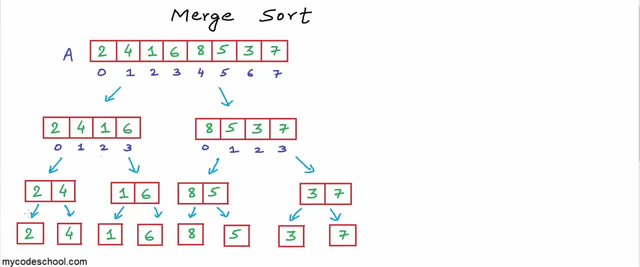 We do not need to do anything to sort it Now. at this stage we can start combining back or merging the sub lists, So these two sub lists can be merged. Let's say we will depict the cells in sorted sub lists in green. We have already discussed the merge logic. 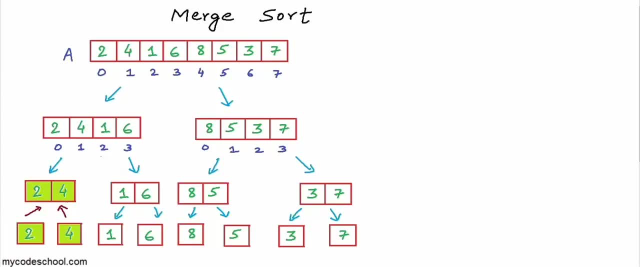 This sub list two, four will still be the same after merge. also Sub lists one and six. these two sub lists with only one element each will also merge. and now we can merge two, four and one, six. Coming to this side, all these sub lists with just one element are already sorted. 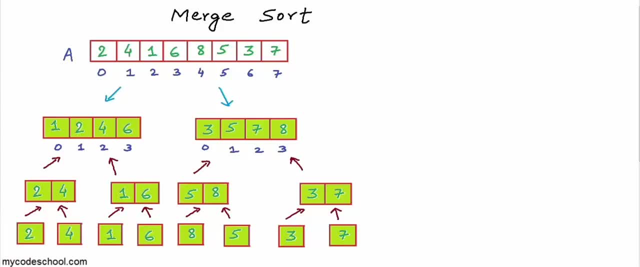 So we will start merging back. Finally, these two sorted sub lists- one, two, four, six and three, five, seven, eight- can be merged back into the original list A. And now let's write pseudo code for this algorithm. I will write a function named merge sort that will take an array A as argument. 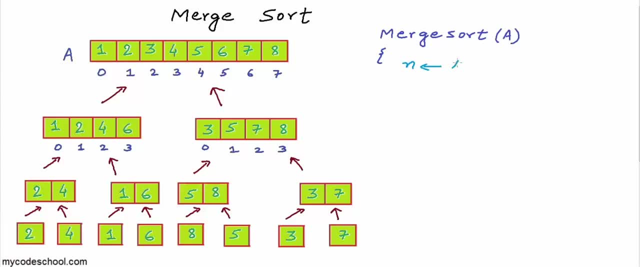 In the function. first I will take a variable that will store the number of elements in A, and now we can partition A into two halves. We need to partition A only if n is greater than one. If n is less than two, then we have only one element in the array. 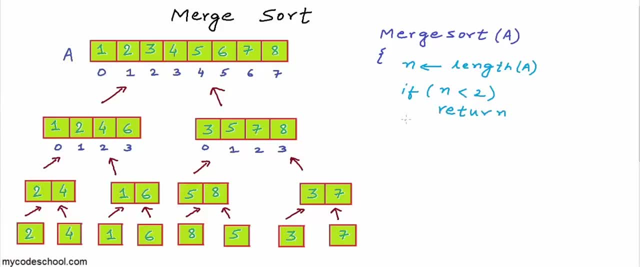 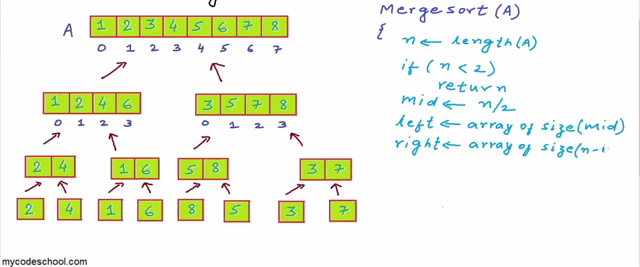 So the array is already sorted. we can simply return. else what we can do is we can first find out a middle position And then we can create two arrays, one of size equal to mid and another of size n minus mid. So first array will have all the elements starting index zero till n mid minus one. 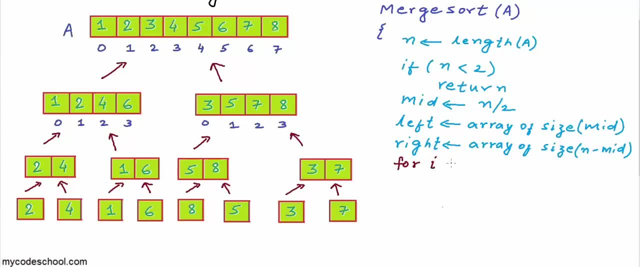 we can just fill the elements. we can run a loop from zero to mid minus one, So there will be mid elements in all and we can say: left i is a i and then we can run another loop from index mid till n minus one. 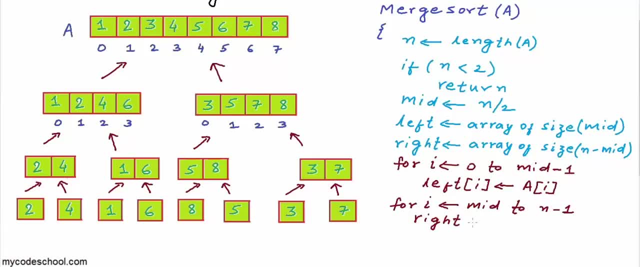 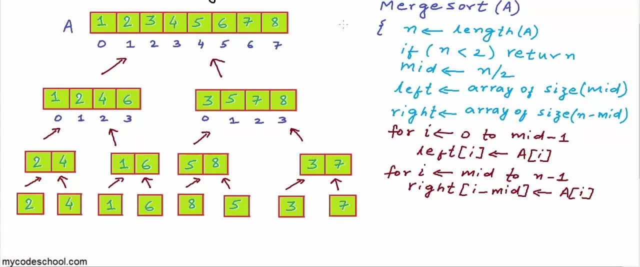 So there will be n minus mid elements in all and we need to fill in right i minus mid as a i. Now that we have created left and right sub lists, we can first make a recursive call to sort the left sub list And once we are done sorting the left, 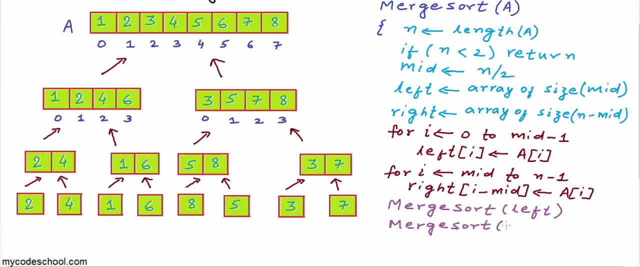 sub list, we can make a recursive call to sort the right sub list And once both left and right sub lists are sorted, we can make a call to the merge function that we had written before to merge left and right sub lists into a 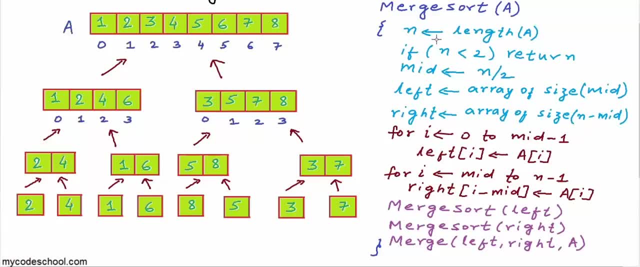 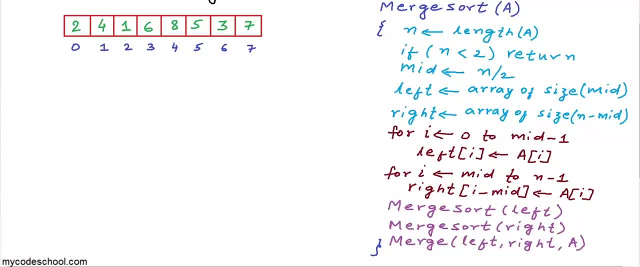 It's really important to visualize how this recursion will actually execute. Once again, I'll start over with an unsorted array And let's say this array is passed to the merge sort function. Now we can see that. Now let's run through this code and see what's happening. 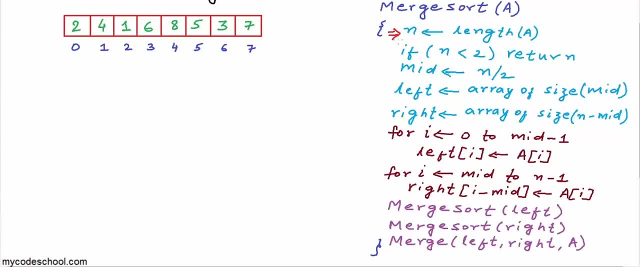 I'll start with the first line. We calculate n, the number of elements in the array. The number of elements in this array is eight. It's not less than two. This condition is not true, So we will not return and exit from this function. 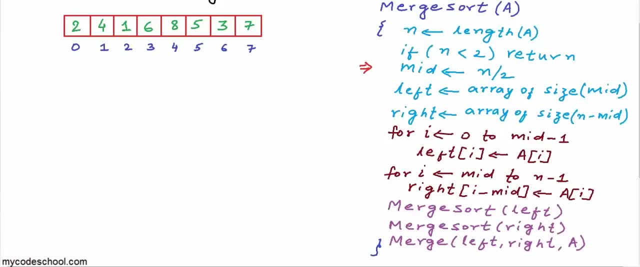 We will move forward. We will calculate the mid index. Now n is eight, So mid will be four. And now we will create two arrays, Left and right, One of size mid and another of size n minus mid. We will fill up these arrays. 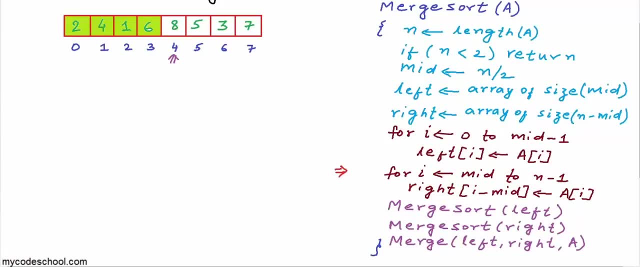 The first four elements will go to left and next four will go to right, And now we are making a recursive call. when a function calls itself, Then such a call is called recursive call. A function calling itself is not much different from a function: a calling another function. 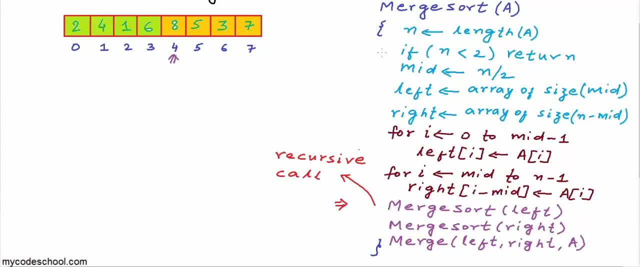 b, At this stage, the execution of this particular function call With this array with eight elements as argument is paused And the machine says that hey, let me go and finish this particular function call and then I'll come back to you. The machine goes on to execute merge sort on this particular array with four elements. 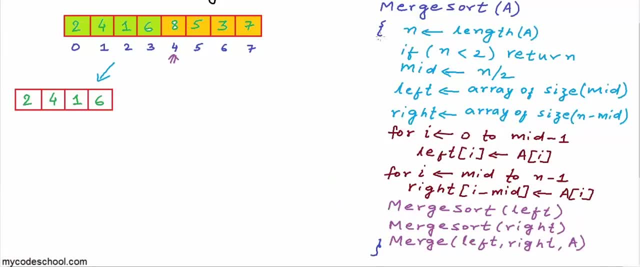 two, four, one and six. Now, once again, we start at the first line in a new call to merge. sort for this new array, n is not less than two, So we will not return and exit This particular condition. n is the base condition or the exit condition from the recursion. 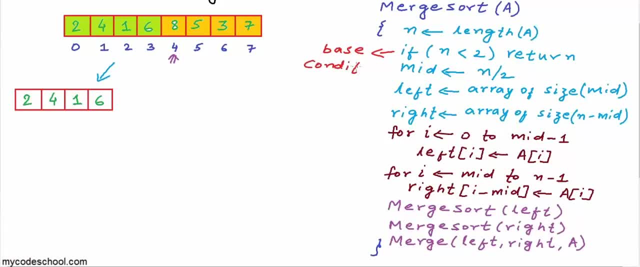 If this was not there, we would have gone endlessly in recursion. We needed to stop somewhere. Once again, we will create lefts and rights And once again there will be a recursive call passing this array to four as argument. So once again, the state of execution of this second merge sort will also be paused. 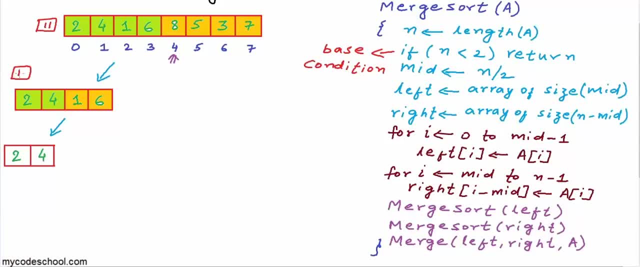 All of these are paused. the state of execution of these functions. the function calls with these arrays as arguments. Now, once again, here also, we will have a recursive call, Now for this particular array with just one element. this base condition will be true. 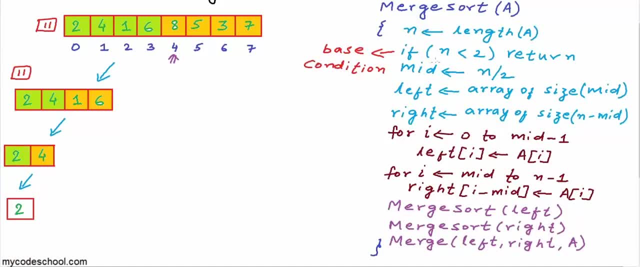 So this call will simply exit. And now for this guy, this array with two elements, two and four, this second recursive call will be made with just this element four which, once again, is the base condition. And now, once both the merge sort, both the recursive calls for this particular state, 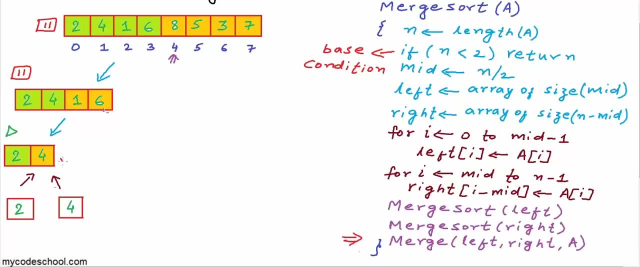 this particular sub list with two elements: return back, merge function will be called And then this guy will finish and then will the control will return back for execution of this particular sub list 2416.. And this guy will make the second merge sort call. 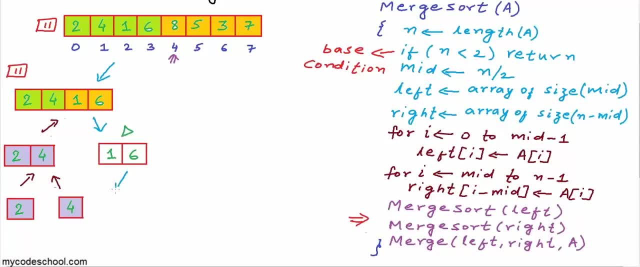 This guy will first make a call for this sub list with just one element, And once this is done, it will make another recursive call. Now we will have a merge for this guy: 16.. And then control will return back here to this array 2416..